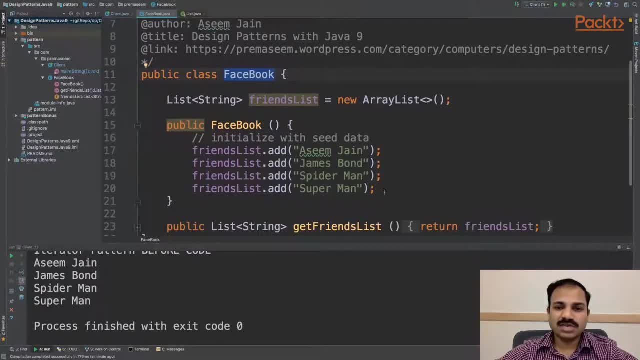 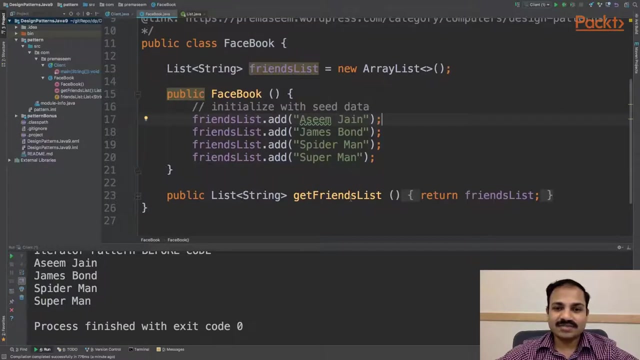 friend list. So in the constructor I have initiated with the seed data, wherein we have all superheroes like James Bond, Spiderman, Superman. Well, I am also there and I am no less than a superhero. No, just kidding. So what we are doing here is we are exposing a getter for this friend list and then the 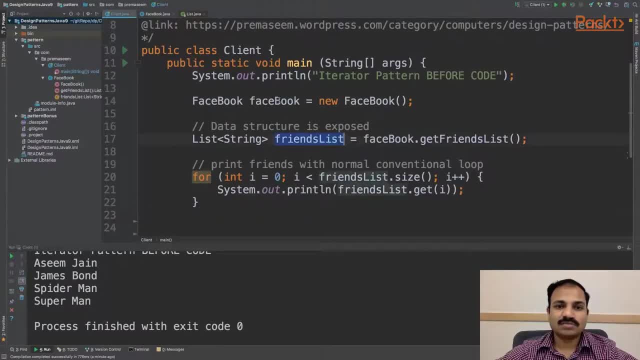 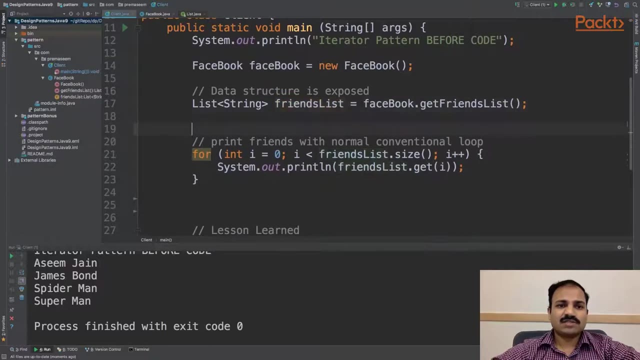 client is getting a hold of this friend list from the Facebook And we are just doing the normal conventional for loop and printing this So it looks simple. They're like: so far, so good. But the problem could arise once someone start modifying the friends list and 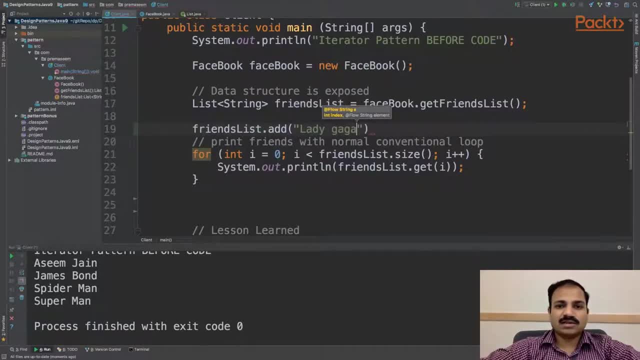 started compromising. So let's say there is a friend called Lady Gaga, a person which I don't want, And then if we run it, we see that one more friend has been added in our friend list, which is Lady Gaga, which is unintentional. 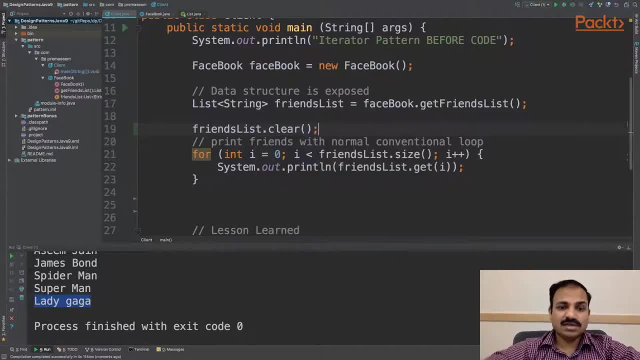 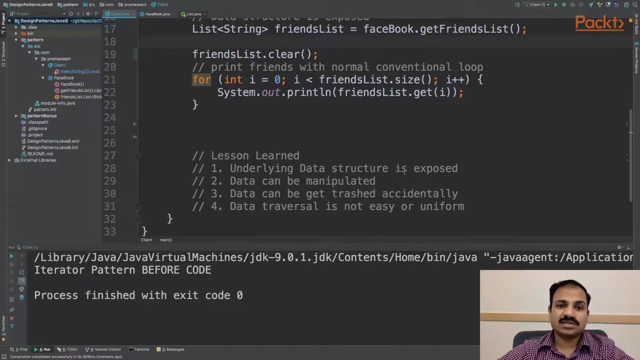 The worst part is if someone accidentally clean- like clear- your data and then it's a nightmare. So what we learned here is, if we expose our data structure directly, underlying data structure is exposed, it's manipulated, it can be trashed accidentally and data traversal is not uniform. 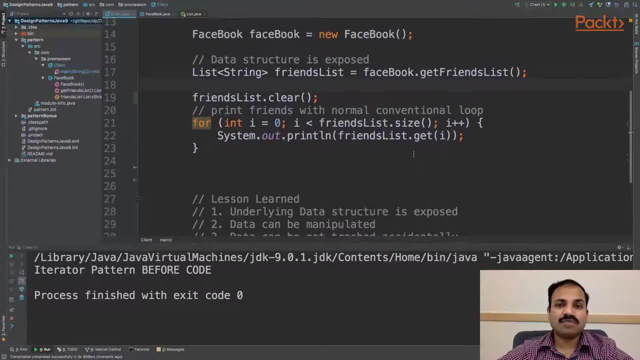 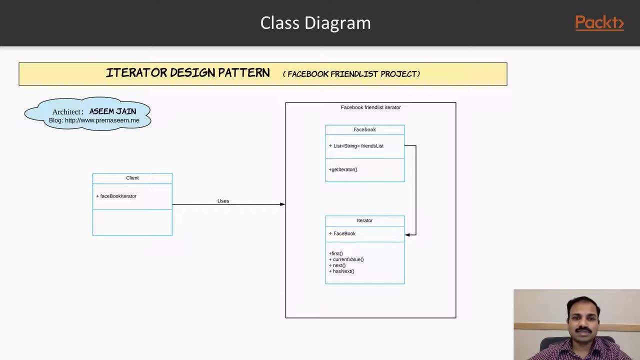 So now let's try to apply iterator design pattern to solve all these problems. So, after refactoring and applying iterator design pattern, our code would look something like this: We are inclined, instead of directly exposing the data structure, we can apply iterator structure will use the iterator. so Facebook class will expose the iterator. 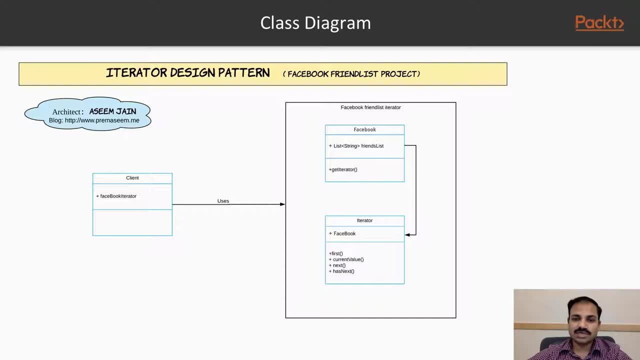 so there is the iterator, which would be the interface, and then it would expose the elements with these methods: first, next has next and current value, which would eventually be used by the client to access the data, and it will have the controlled access. let's look at the sequence diagram wherein client gets the 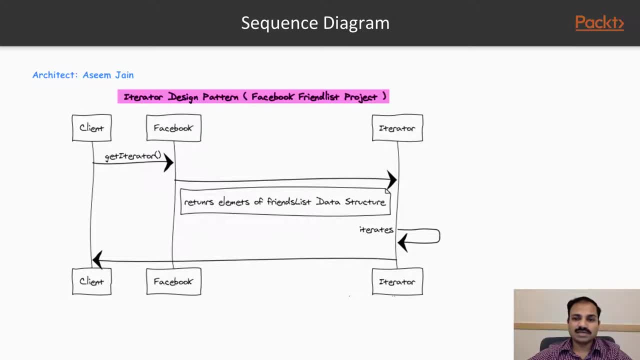 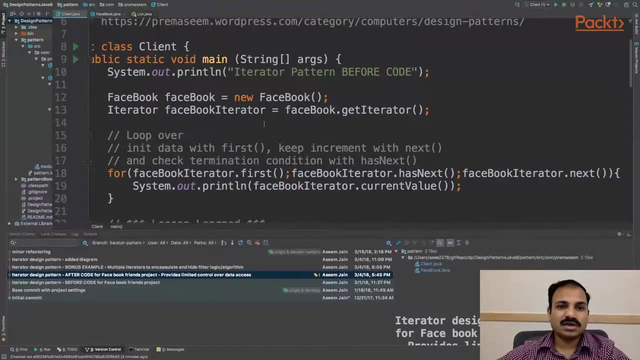 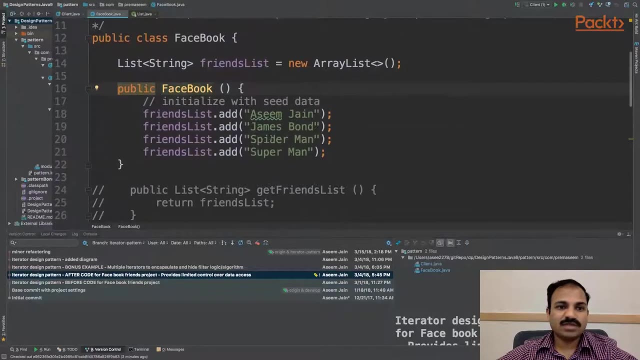 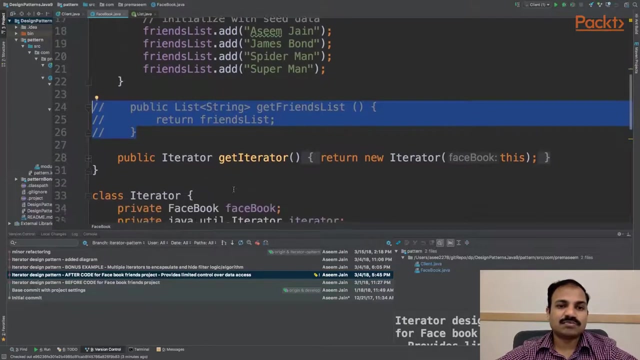 iterator from Facebook class and then it start iterating element by element and that's what gets printed in the client. here is our updated code. so let's look at the Facebook class. we have the same data, but friend list. we have removed the getter, so we don't expose it directly, but we are exposing it through the. 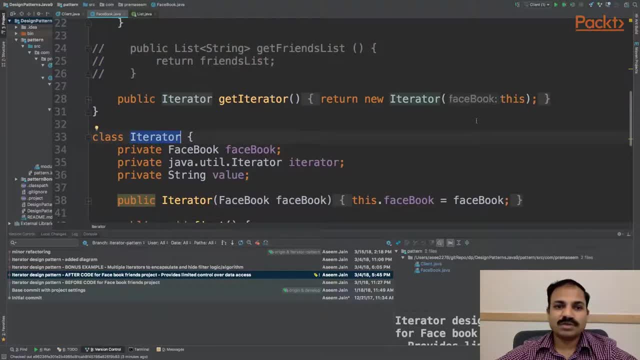 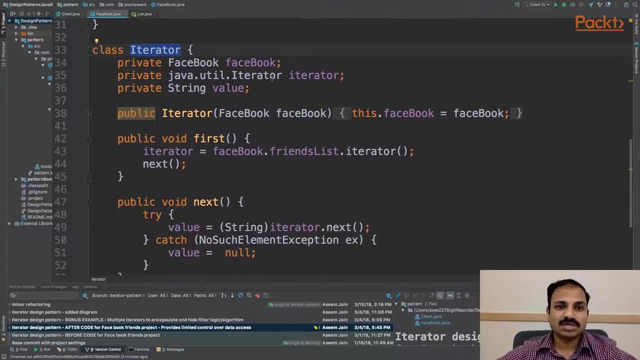 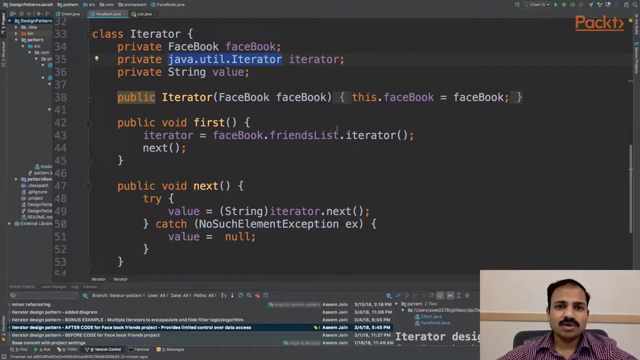 iterator. so we have iterator class here wherein we pass the Facebook. now Java provides us the default iterator implementation in the list by Java utils iterator. we are just using that here. so what we do here is that from the list, once we call iterator, it returns us this: 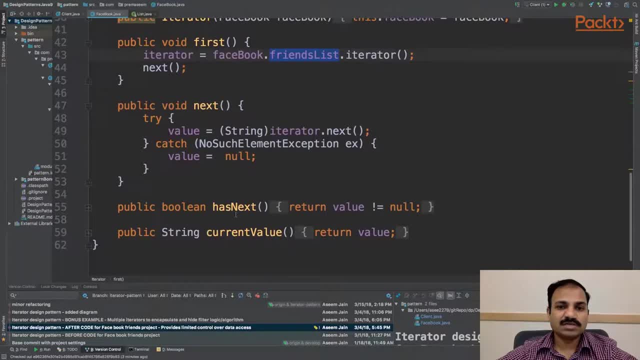 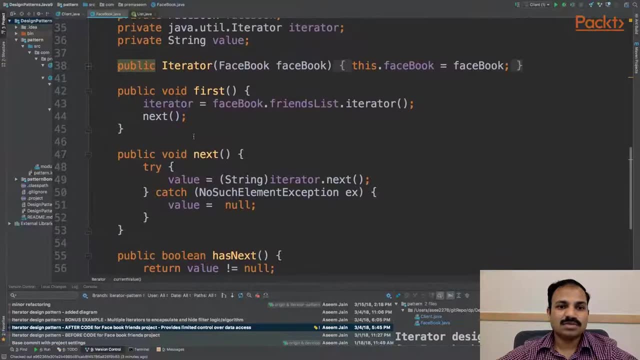 iterator, and then we expose our internal methods which uses that iterator to give us the sequential access of the iterator. and then we expose our internal methods which uses that iterator to give us the sequential access of these elements which ultimately get used by the client. so it looks something. 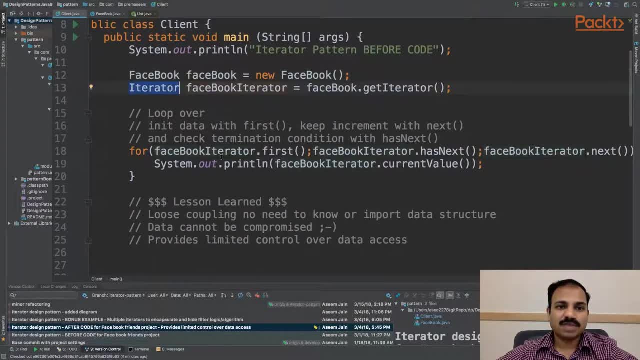 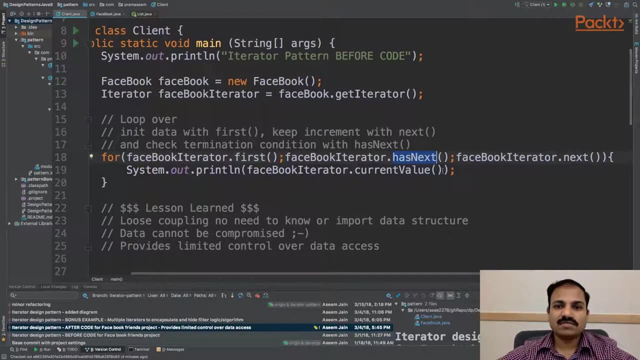 like this here that we get the iterator and then we call the first like initial data with the first in a data with the first, keep increment with next and check termination condition it has next. so till the time it will have the data, it will iterate over and keep printing the current value. so lesson learned is loose. 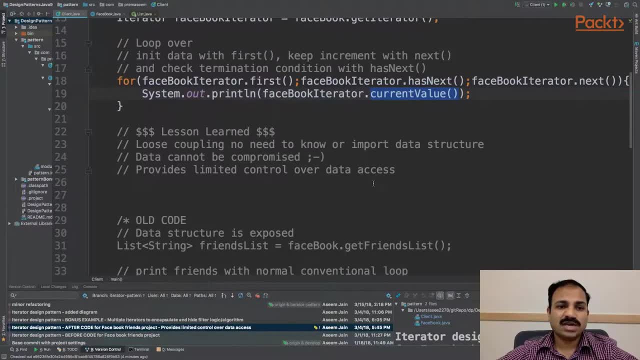 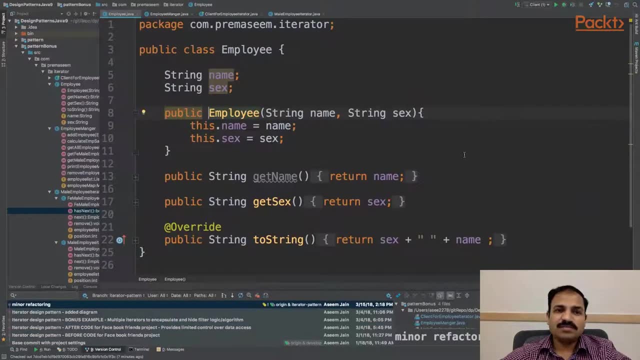 no need to know or import data. structure. data cannot be compromised. provides limited control over data access. as part of bonus example, let me walk you through another iterator implementation. but you need to check out the code and dig deep to understand it better and quickly go through it. so we 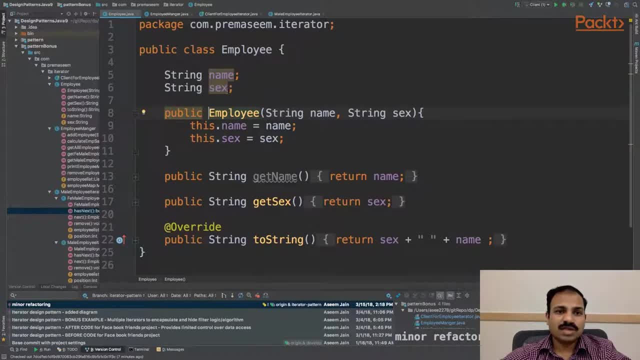 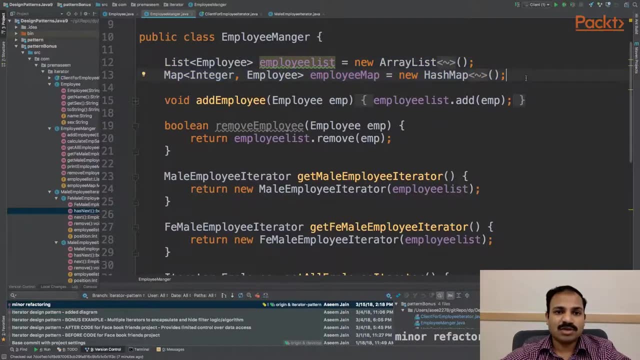 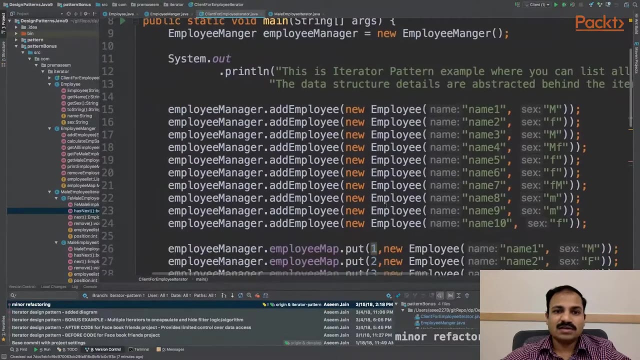 have an employee class which is just a normal pojo with names and other fields. then we have an employee manager which holds the data in two data structures are employee list and a m-fi map. so here is our client. now in our client we try to add the data in the employee list and then also with the